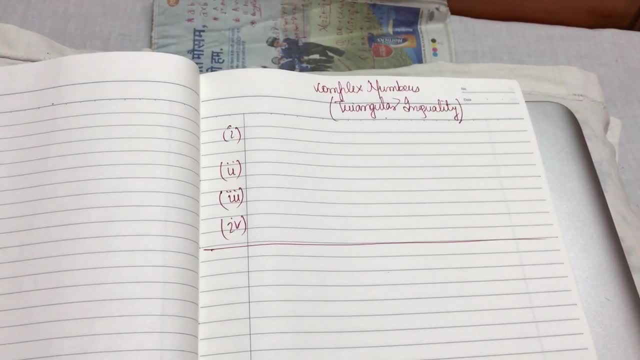 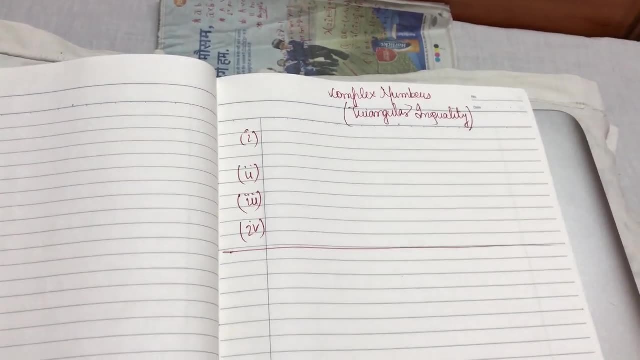 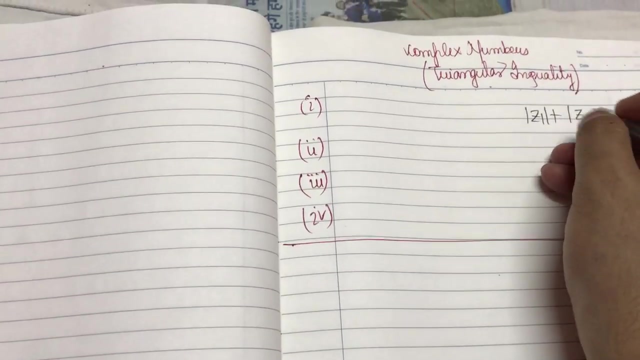 Hello friends, in this video I shall be taking the complex numbers: triangular inequality. Okay, so first of all I would like to begin with how to remember the inequalities. So let's begin. So right here: z1, mod of z1 plus mod of z2.. In the second part, also write this: 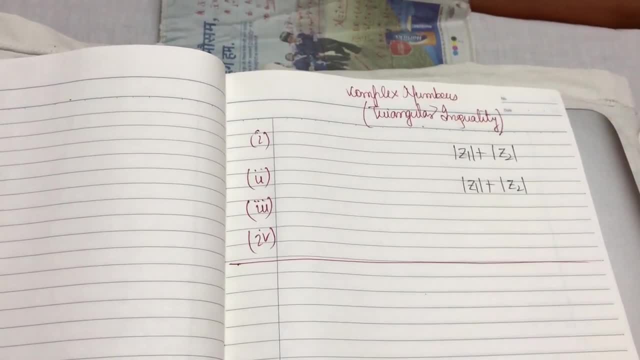 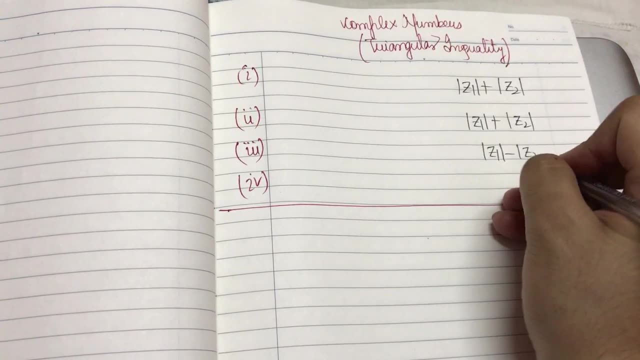 mod of z1 plus mod of z2.. Now in this third and the fourth part we have to take the negative signs, So mod of z1 minus mod of z2.. Now I'm taking the whole mod here. I'll tell you the. 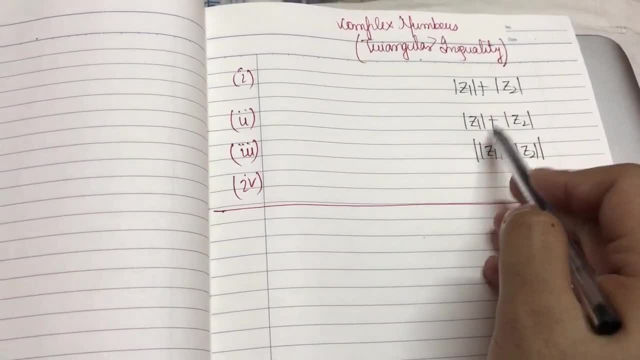 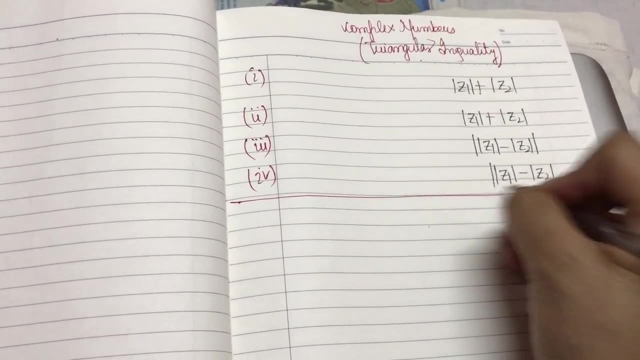 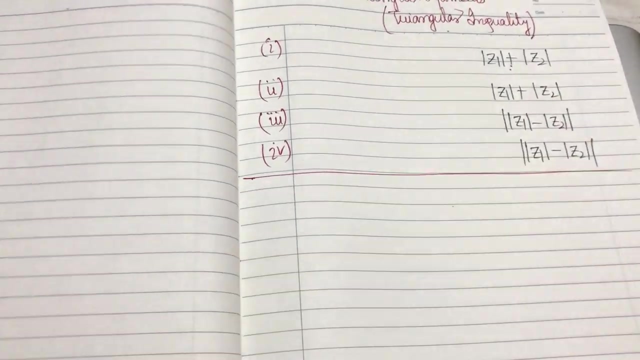 reason later on. But first of all you must remember I'm taking the positive sign in the first two cases and the negative sign in the next two cases. So mod 1, mod z1 minus mod z2, whole mod. Okay, so whenever I'm having the plus sign in middle I have to take the greater than. 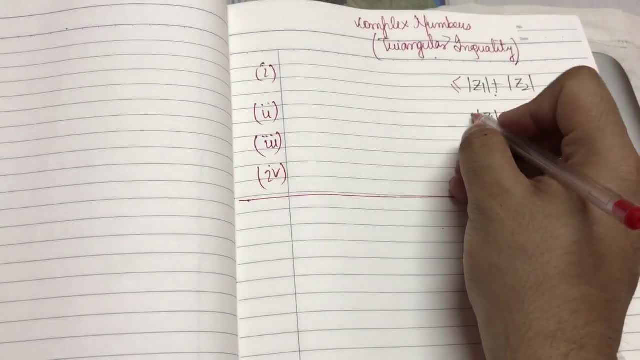 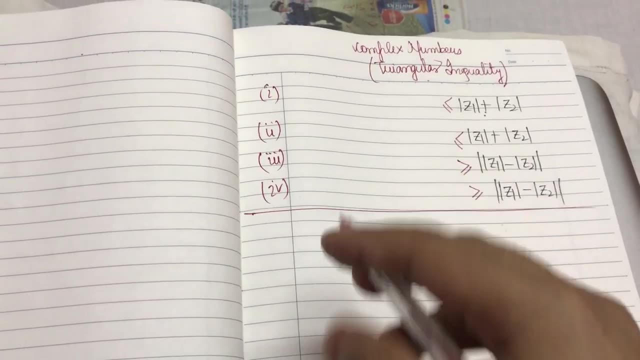 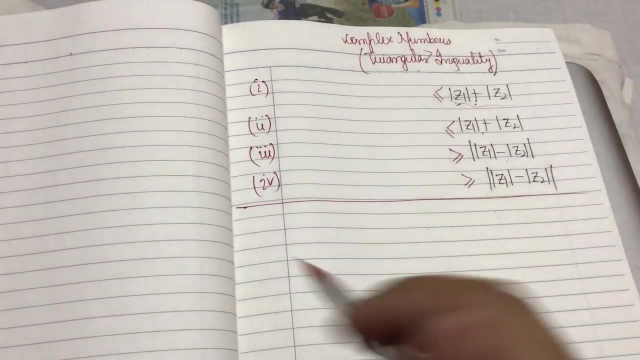 equal to sign. So greater than equal to, greater than equal to. And here, whenever I'm having the negative sign less than equal to, less than equal to the signs I'm taking with respect to this side. Okay, so the positive sign, positive sign, negative sign, negative sign. So I have only two cases to decide, that is z1 plus z2, whole mod. 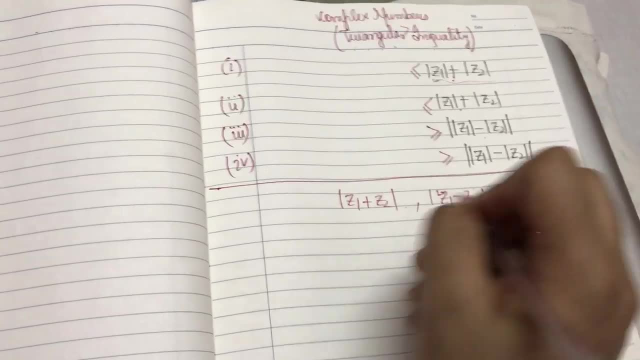 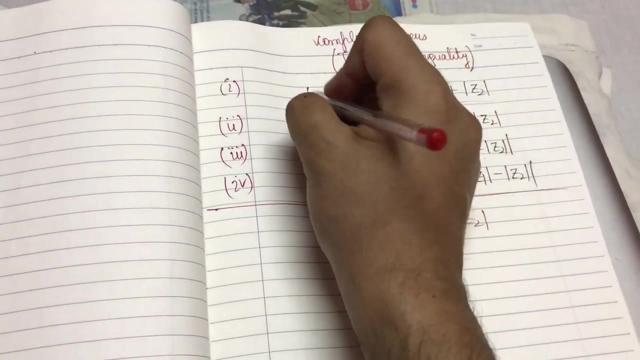 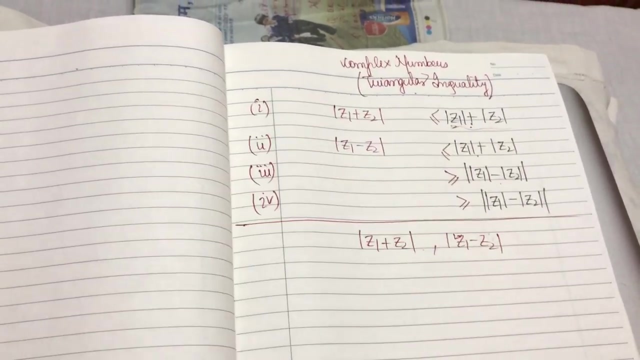 and mod of z1 minus z2.. Okay, so we have to just fit this cases alternately: in these cases in the mod of z1 plus z2.. Then in the next case, mod of z1 minus z2, in the next case, mod of z1 plus z2. and. 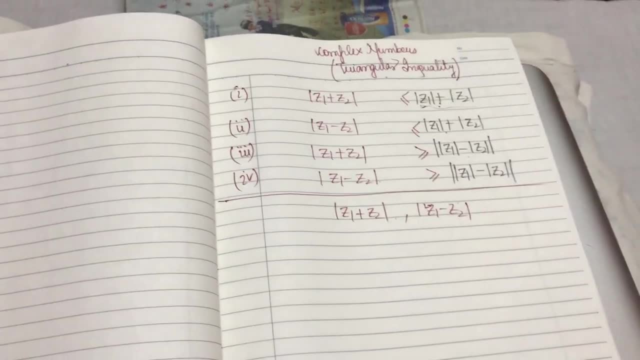 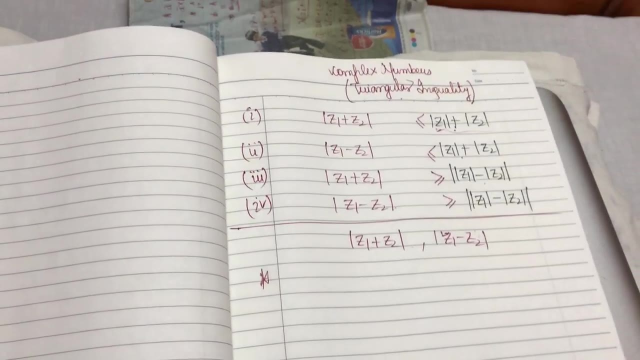 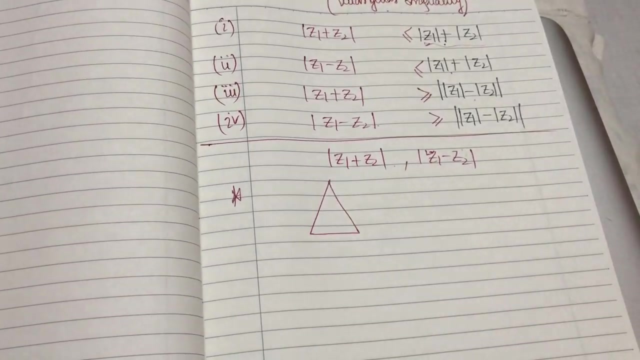 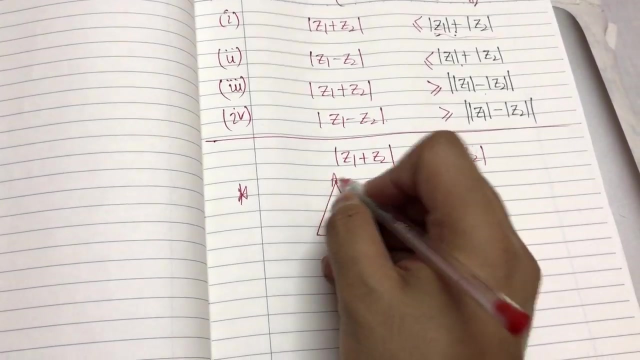 then z1 minus z2.. These inequalities are derived from a triangle, So these are known as the triangular inequalities. I will just prove one unique inequality for the sake of completion. The rest you must have studied. So, like I have a triangle, okay, so the vectors actually behave. Sorry, the complex numbers actually behave as vectors. You. 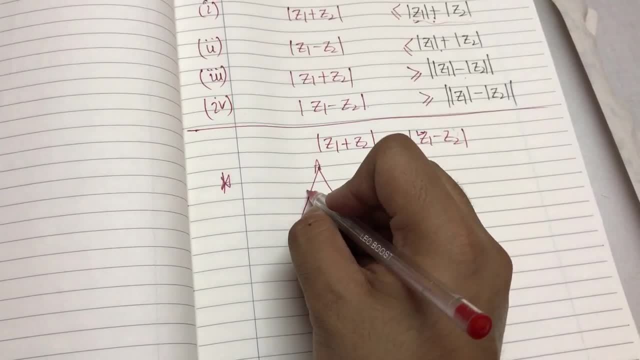 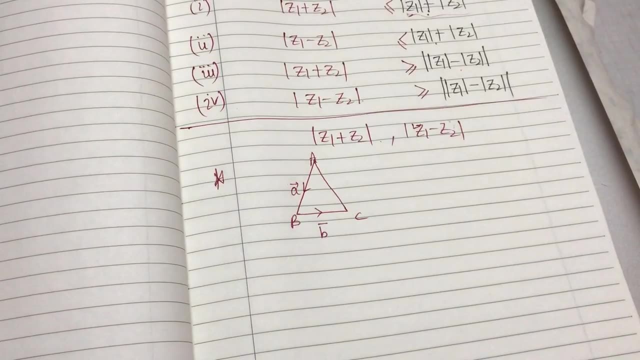 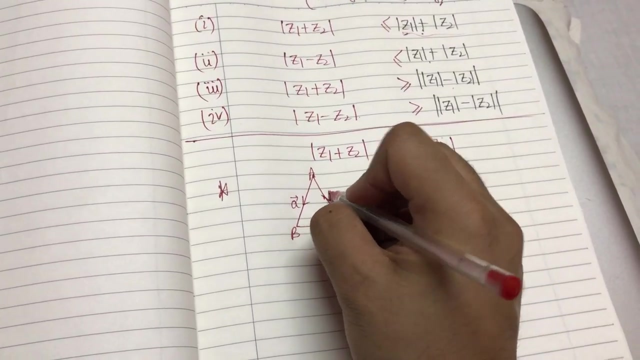 would come to know. If I, if I take this as a, b as a vector and b vector, then what will be the resultant? I think you must have figured, net is so the resultant will be this side, okay, So basically what I'm writing, that 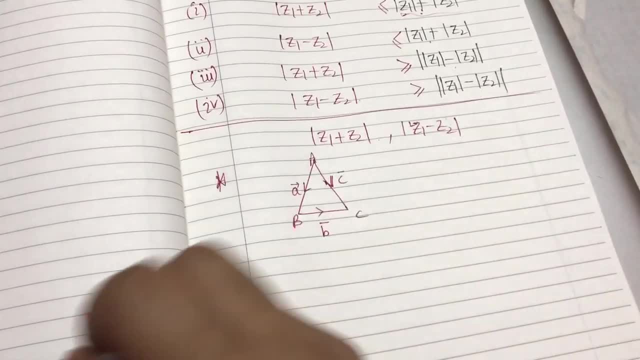 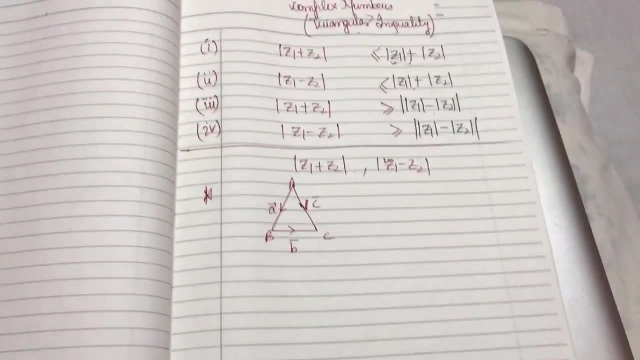 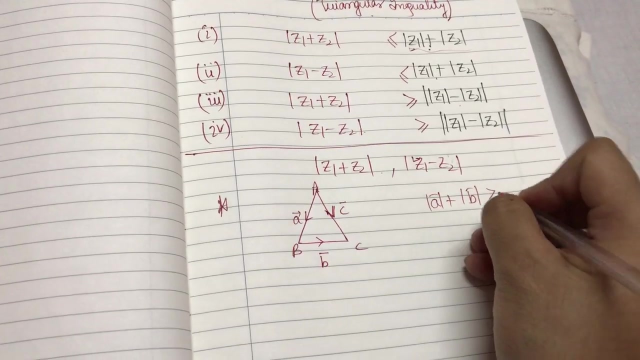 bar plus b bar is equal to c bar in the vector form. okay, so you must. you must be knowing that the sum of two sides must be greater than equal to the third side. so the sum of two sides will be must be greater than equal to the third side. so what? what is basically c? c is equal to a bar plus. 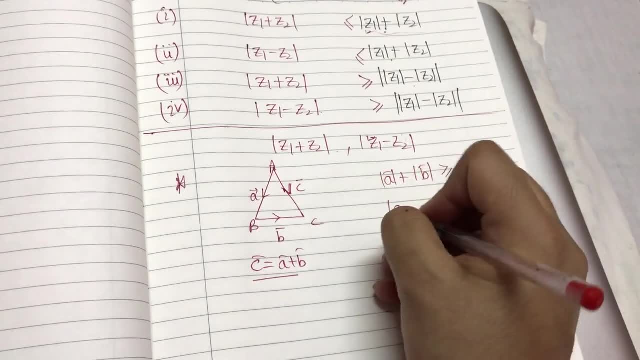 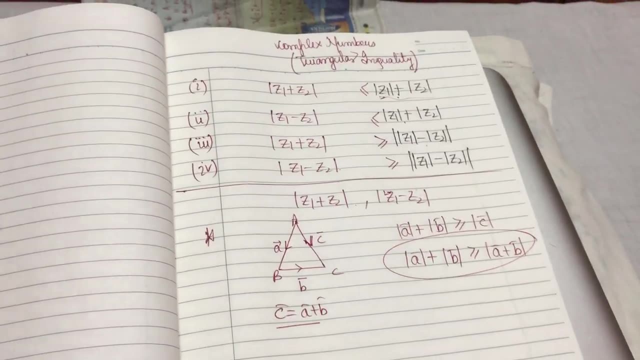 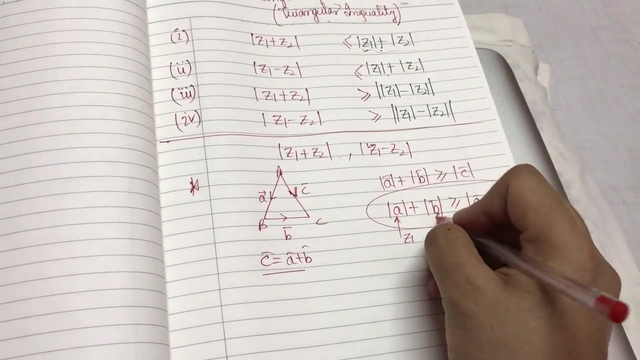 b bar. you must have showed it in the vectors. so mod of a plus mod of b must be greater than equal to this thing. okay, so here is one proof for what we can write in the triangular inequality. you can just replace this by z1 and z2 and so on. so this is the basic, the basic proof for the complex number. 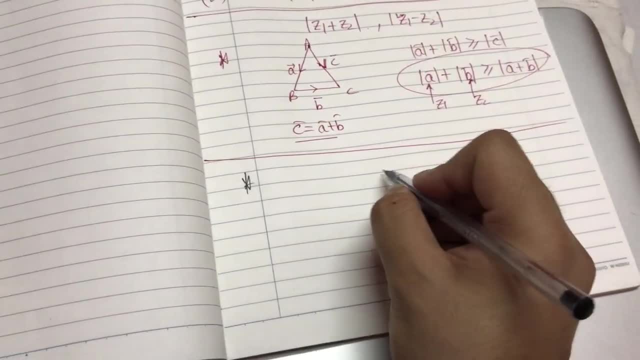 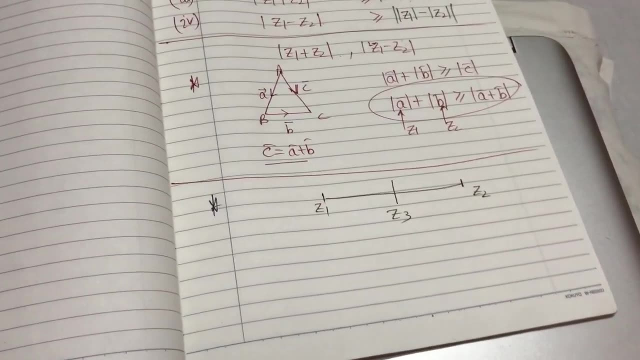 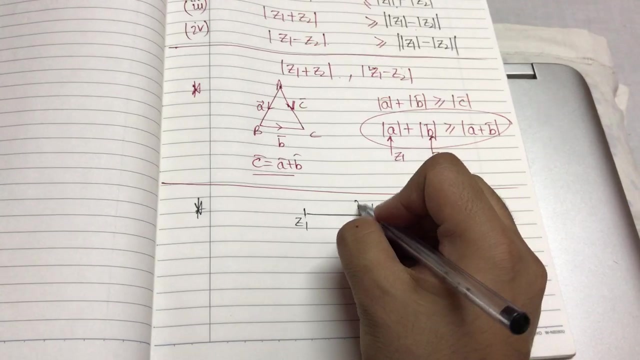 triangular inequality. okay, so now i want to tell you that how to decide whether three complex numbers are collinear or not. two complex numbers will always be collinear, as you started in the straight lines also, so let me take a complex number, z3, that divides z1 and z2 in the ratio m is to n, so now apply the section. 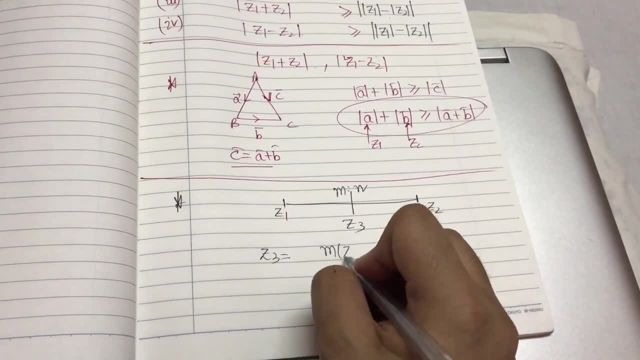 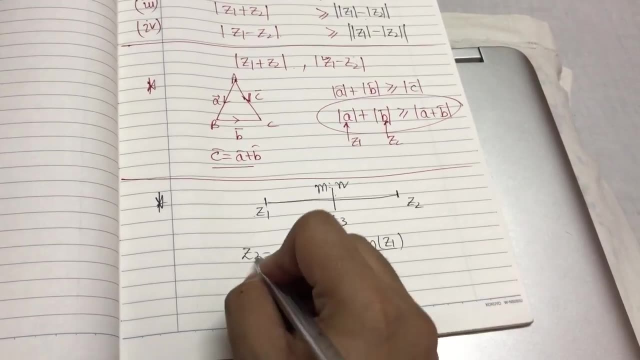 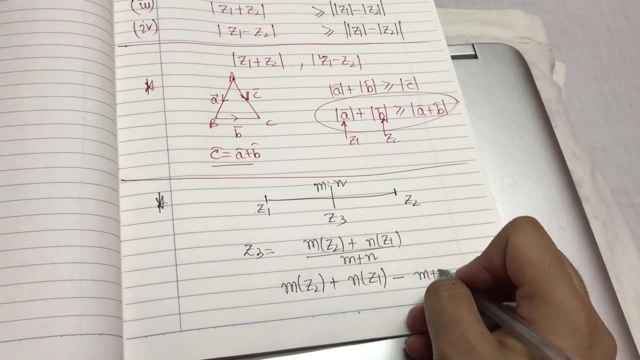 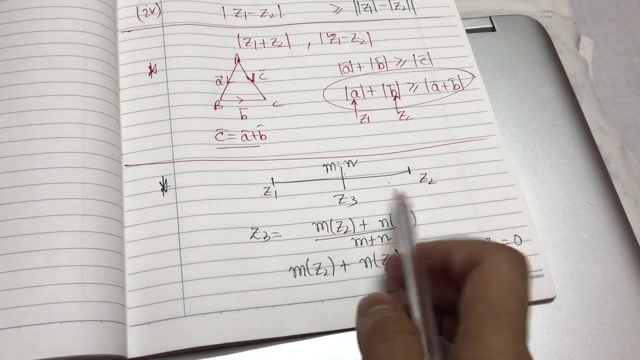 formula. so z3 will be equal to m into z2 plus n, into z1, by m plus n. so take this here. on further calculation we'll get m, z2 plus n, z1 minus m plus n, z3 is equal to zero. you already know that these three are collinear, so whenever 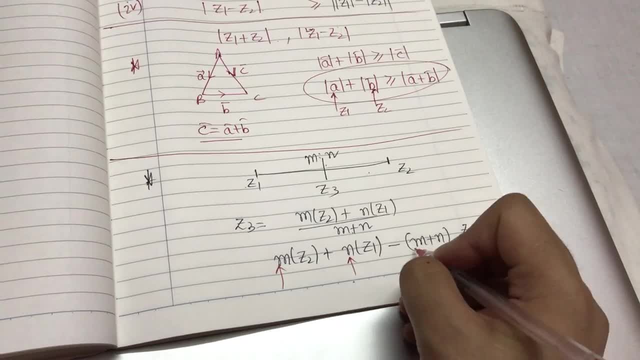 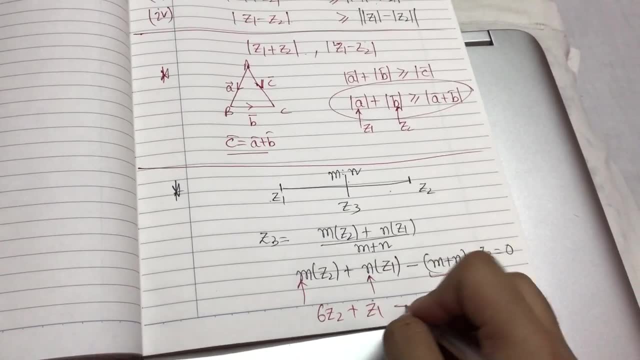 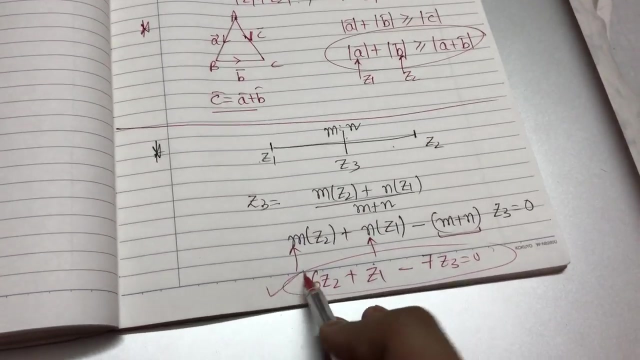 three complex numbers will be collinear, then the sum of the first two must equal to the third one, like 6 z2 plus z1 minus 7 z3 is equal to zero. this question was asked in 2015 bits actually in the paper. if it is directly asked, then it does not strike, so that's why i want to make you clear. 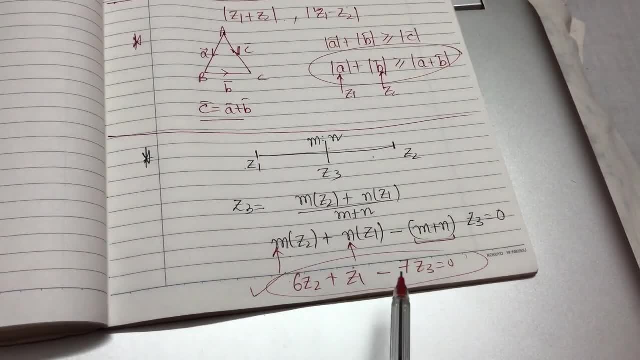 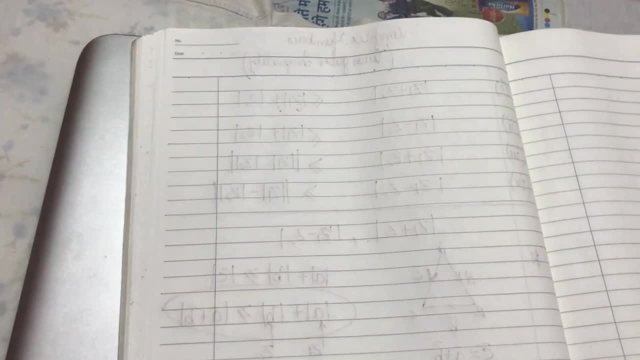 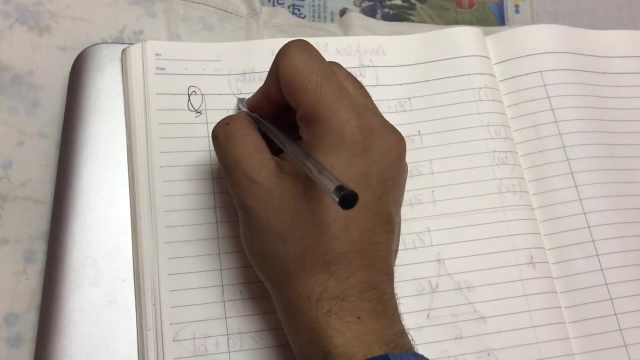 here by using the section formula that these two vectors will be collinear. okay, basically i am saying vectors, because vectors and complex numbers are almost identical. okay, so now i am going to teach you a couple of questions that how to use the triangle inequality. so the first question is: 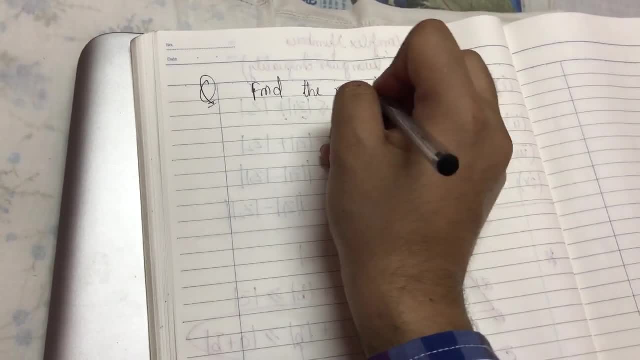 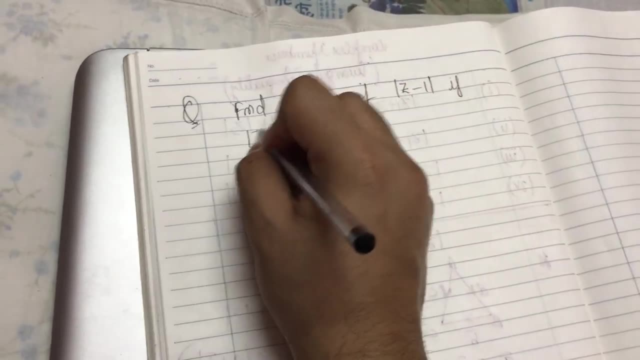 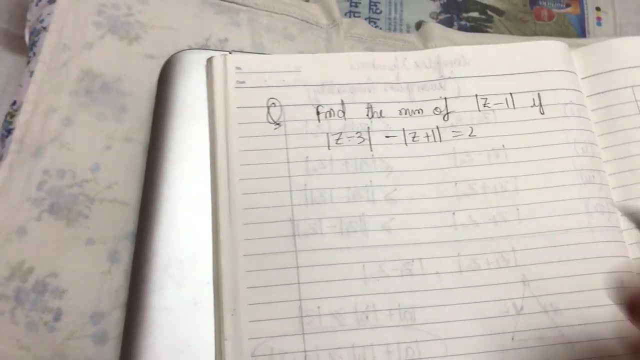 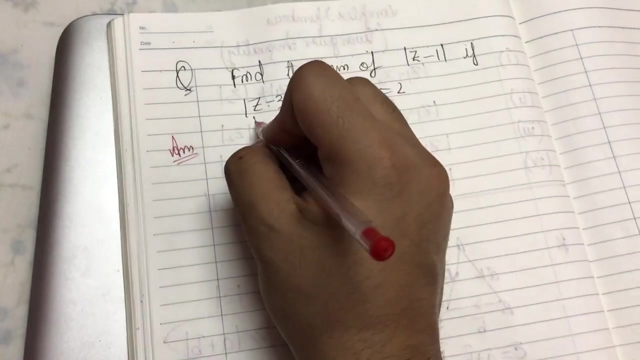 find the minimum of mod of z minus 1. if the condition given is mod of z minus 3 and this mod of z plus 1 is equal to 2, okay, so we have to not fear on seeing the question. so first of all, assume this thing as z1 and this thing as z2, so basically what i am given. 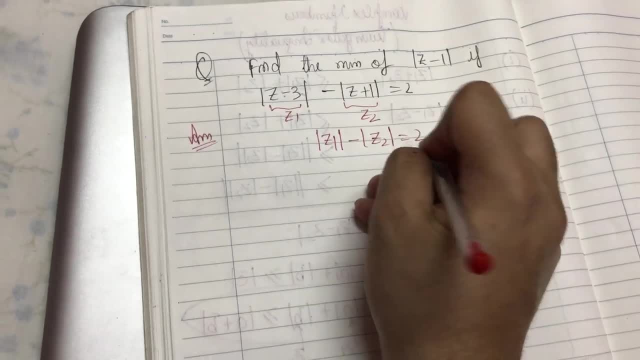 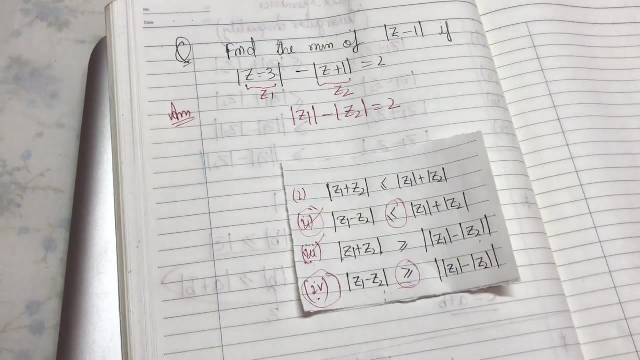 mod of z1 minus mod of z2 is equal to 2. so these are the four inequalities. okay, now decide which one we have to use. we have actually two options here. this is mod of z1 minus mod of z2, so i am having the third option, i am having the. 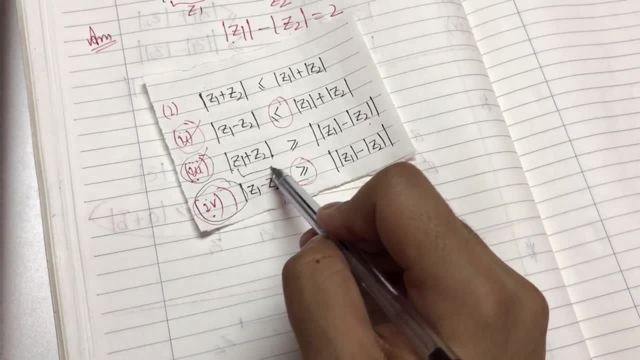 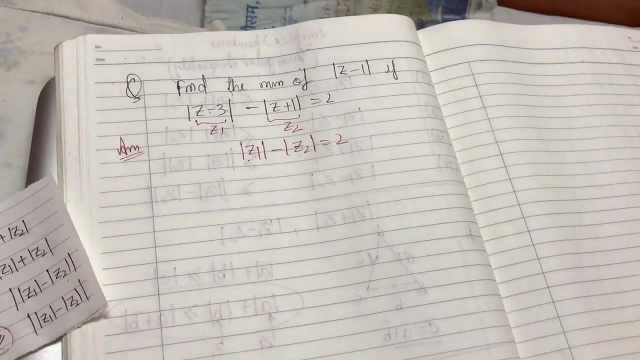 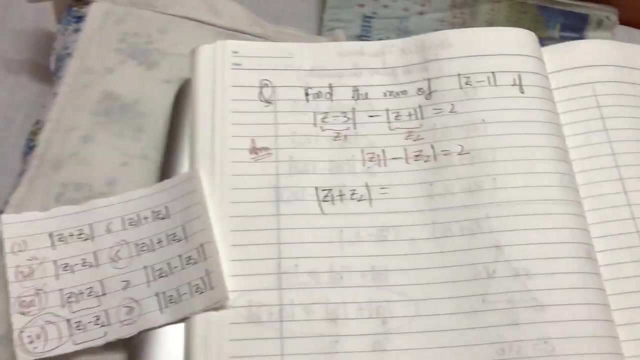 fourth option. so basically, i have to see the lhs, according to which i will decide. so now, first of all, try to get mod of z1. so i want to get mod of z1. just let me write z1 plus z2, whole mod. let me try this one. see, i have two options. so i am trying the third option first. so it will be mod of z minus. 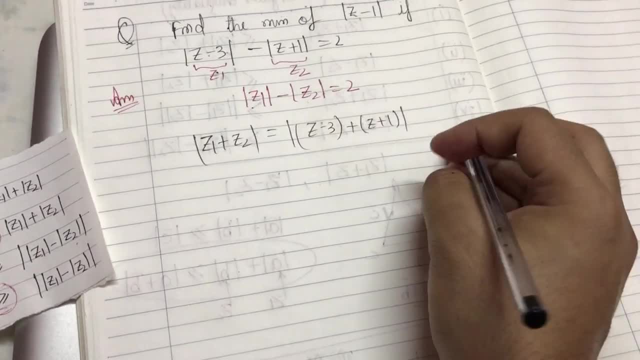 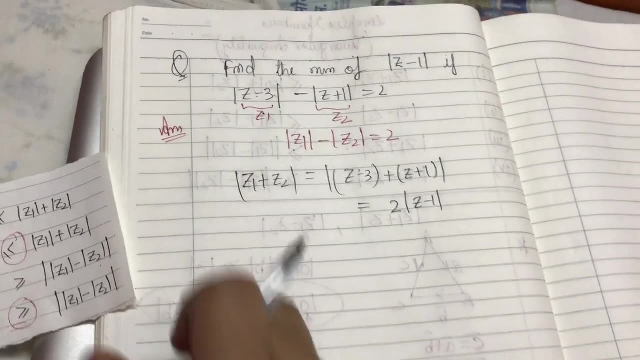 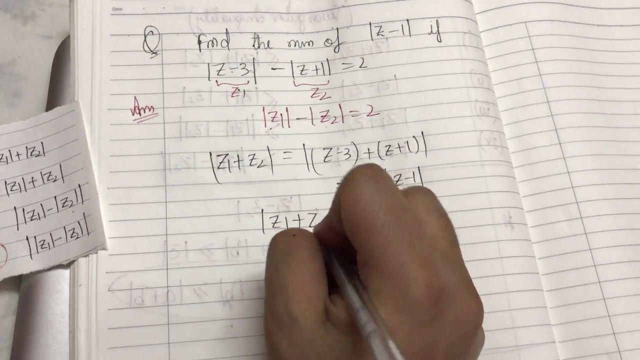 plus z plus one whole mod. okay, so that will basically turn out to be two into mod of z minus one on simple calculation. so you can now. you know now that you have to use the third inequality, so now let's use it. the third inequality says mod of z1 plus z2 must be greater than equal to mod of z1. 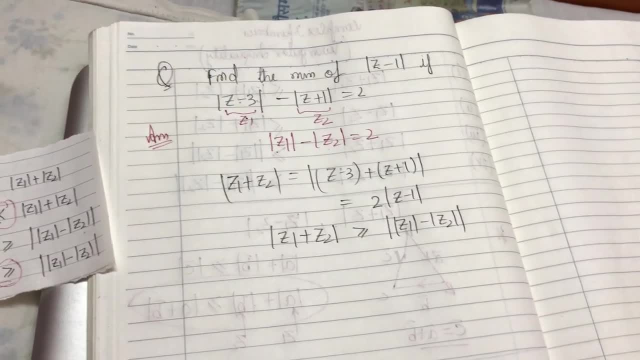 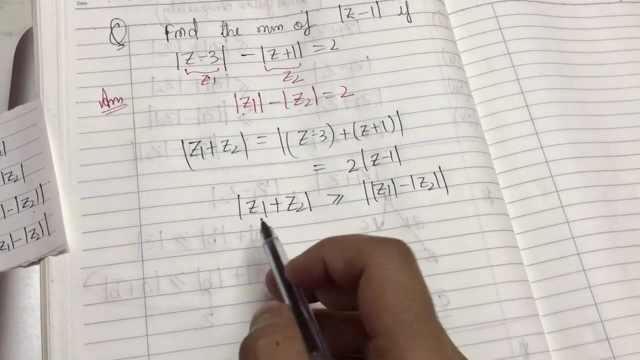 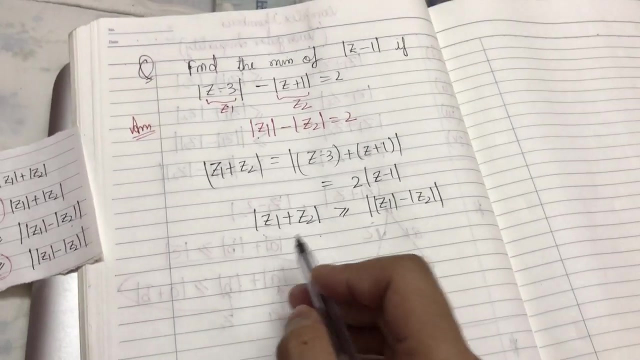 minus mod of z2. okay, now let me tell you why putting the mod outside also. because if i get an equality sign in between, this thing will be positive, so this thing must also be positive. so i am using the modulus outside also. okay, so mod of z1 plus z2 is basically two into. 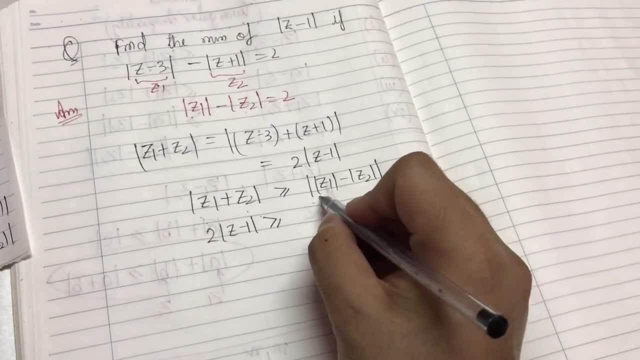 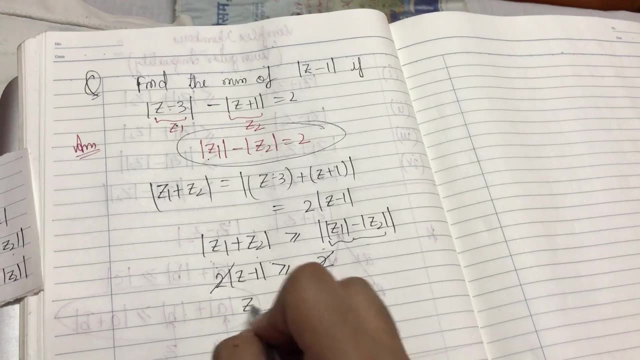 mod of z minus one must be greater than equal to. now, what is this thing? this thing is: two must be greater than mod two. so that is two. so mod of z minus one must be greater than equal to one. so what is the minimum value? that is, 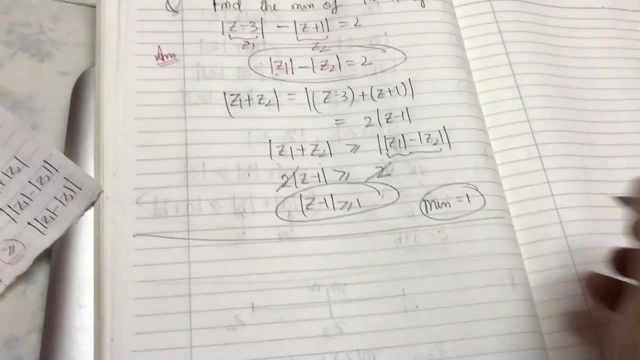 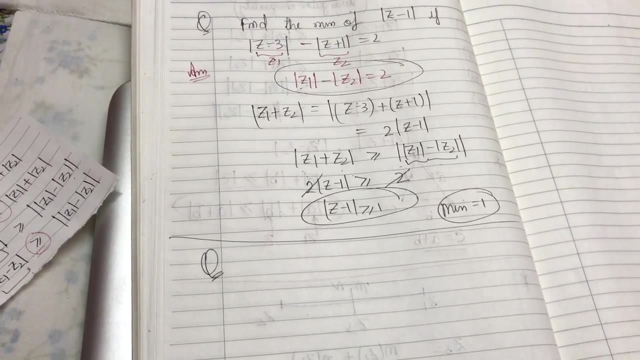 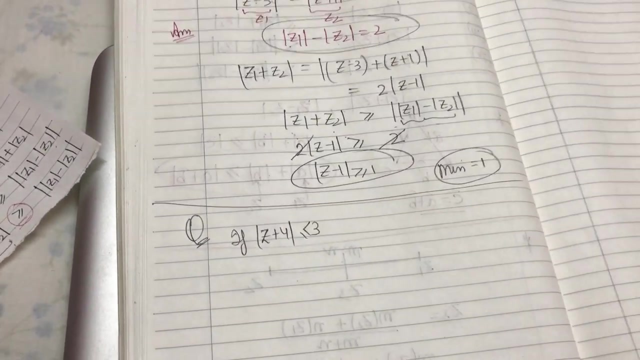 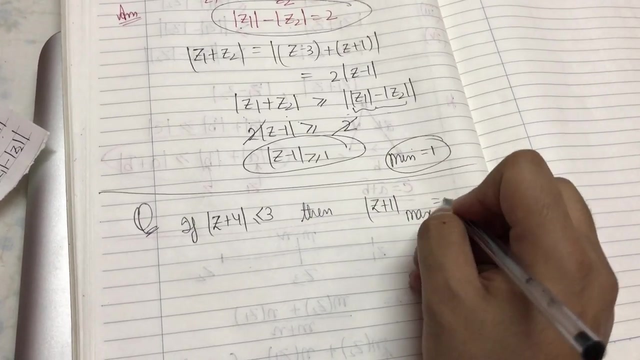 that is one. so, okay, this was a simple question, simple actually, these type of simple questions seem simple, but the concept is very hard to understand. so now the second question. if mod of z plus four is less than equal to three, then i have been asked the maximum value of z plus one. okay, so these are the four triangular. 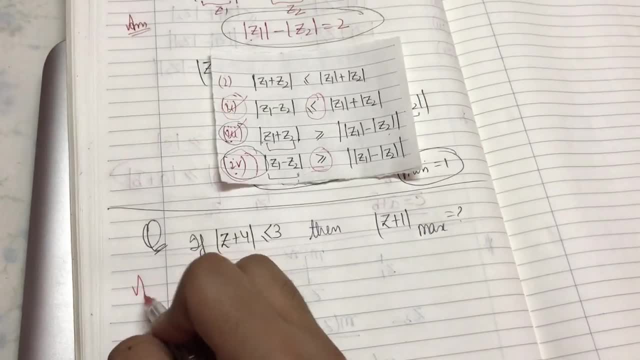 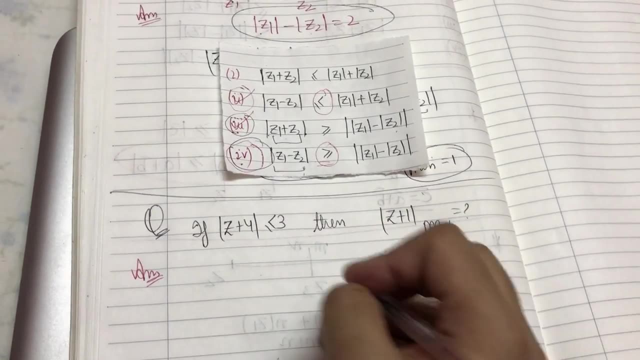 inequalities that i have now let me solve it. let me solve it. i have been asked the maximum value of mod of z plus 1, so first of all i have to derive mod of z plus 1 from somewhere so mod of z plus 1 can be written as: 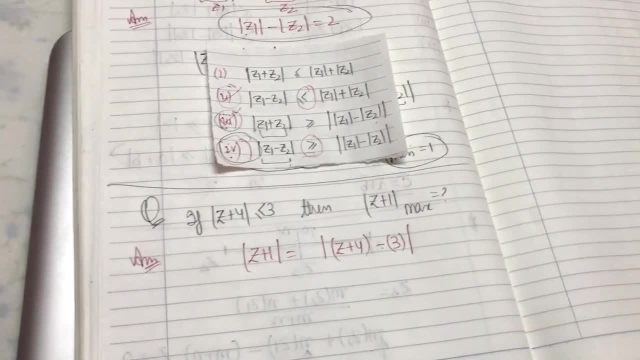 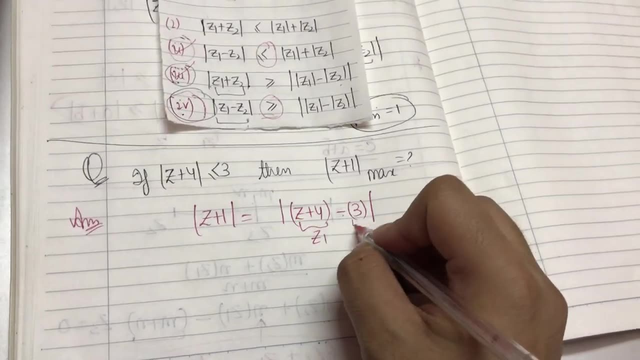 this thing minus 3. okay, i can write this as this, so let me take this as z1 and this is z2. the real numbers are also complex numbers and z1 will be a the nth 연�. Thank you for watching and i will see you in my next videos. receive good health etwa. 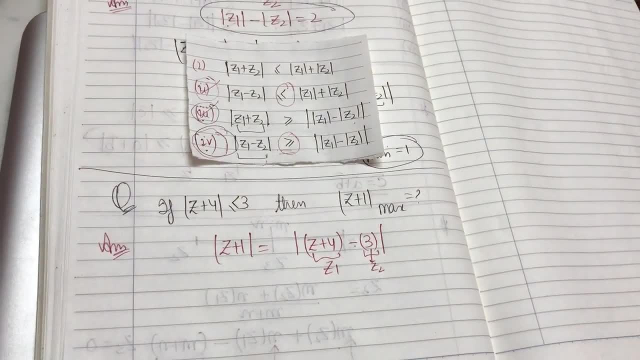 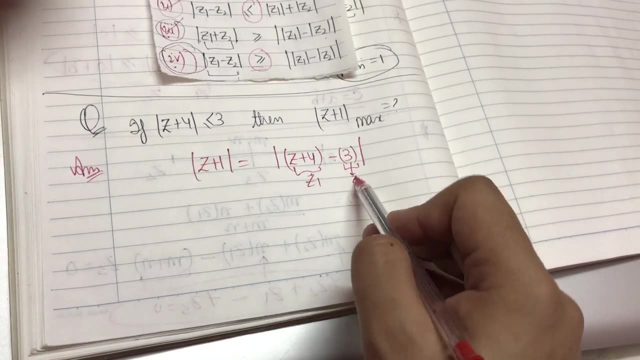 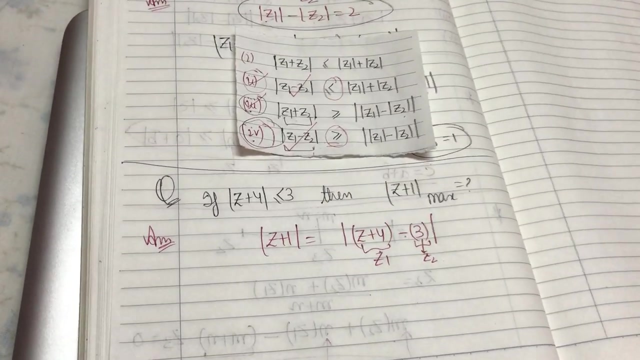 the real numbers are also complex numbers. complex numbers with the imaginary part as zero. so three is also actually a complex number. okay, so i i got mod of z1 minus z2. so which two cases i'm getting? case number two and case number four. so i need to decide further. i have been asked the maximum value. okay, now you're going to tell me. 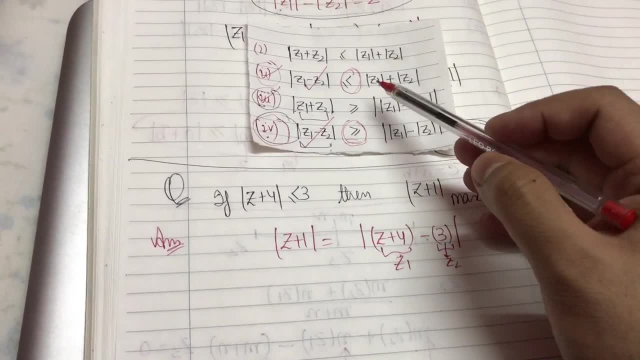 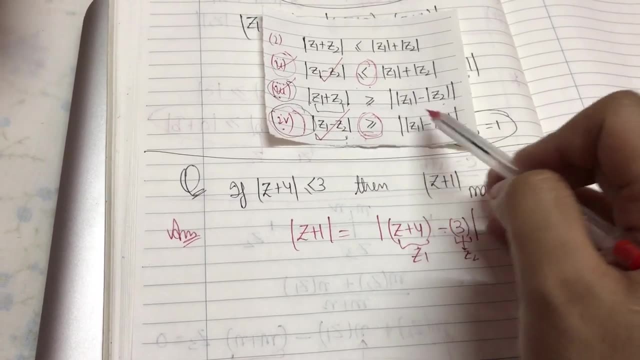 that here i have this sign. here i have this sign. so in this i'll get a maximum value- see- less than equal to. in this i'll get a minimum value. for example, it comes greater than equal to one, so the range will be one to infinity. so the maximum value would tend to infinity. so that is of no use here. 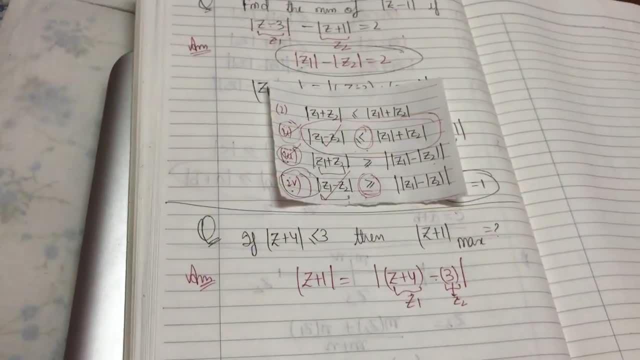 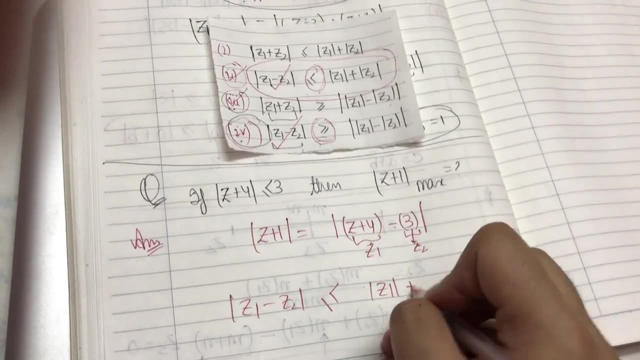 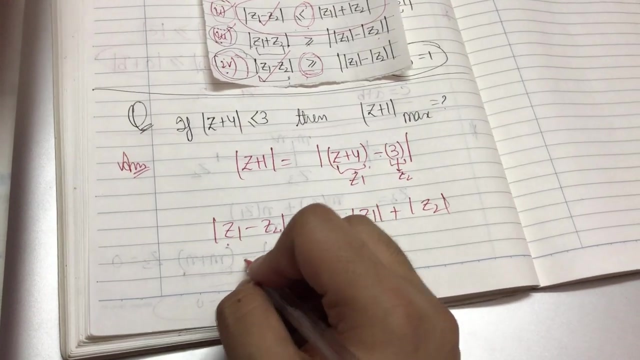 so we have to use the second equation here, so i can write: mod of z1 minus z2 must be less than equal to mod of z1 plus mod of z2. what is mod of z1 minus z2? that is this. so it will be z plus 1.